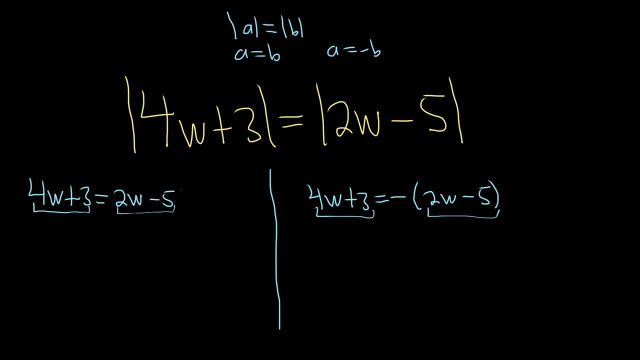 I do a plus and a minus. Okay, let's solve each of these individually. So here we want to get all the w's on one side by themselves, So we'll start by subtracting 2w. So minus 2w, minus 2w. These cancel 4w. minus 2w is 2w. 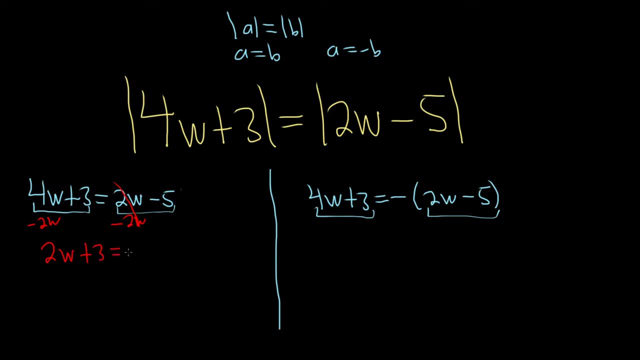 We still have the plus 3, and this is equal to minus 5.. Now we can subtract 3 from both sides, So we have 2w equals minus 8.. Almost there, Our w is being multiplied by 2.. So what we can do now is just simply divide by 2.. 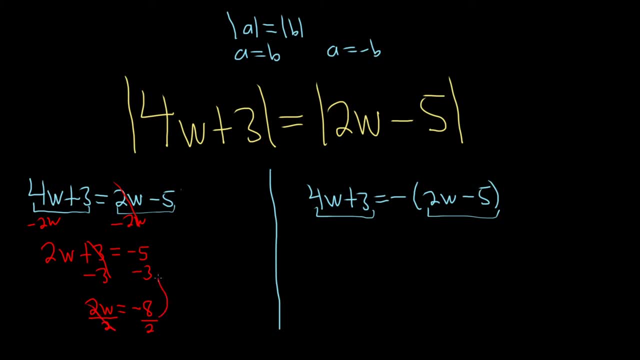 Divide by 2.. And so we have w equals negative 4.. So that would be the first answer to our absolute value equation. Over here on the right, it's very similar. We first have to distribute this negative 1.. So it's 4w plus 3.. 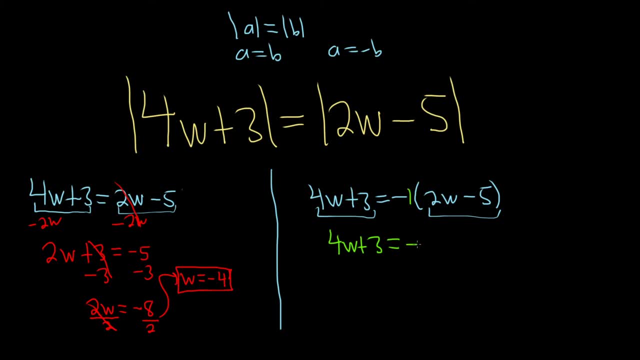 That's equal to- let's see, negative 1 times 2w is negative 2w, And then negative 1 times negative 5 is positive 5.. And again, our goal is to get all of the w's on one side by themselves. 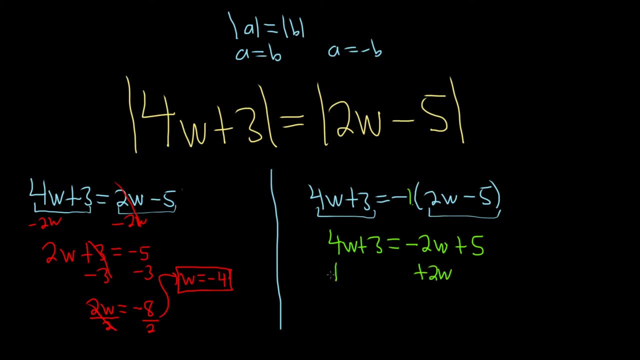 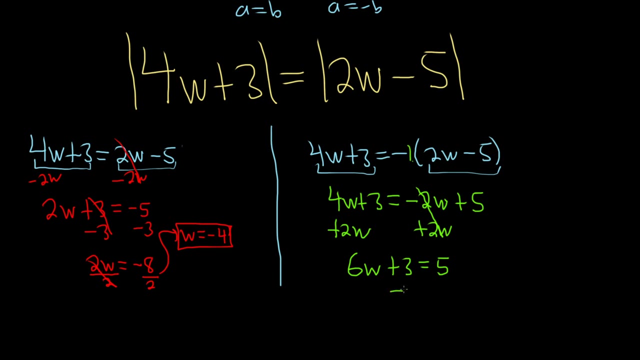 So we'll start by adding 2w to both sides, So plus 2w, plus 2w. These cancel, So we have 6w plus 3, equals 5.. Then we'll subtract 3 from both sides, So minus 3. 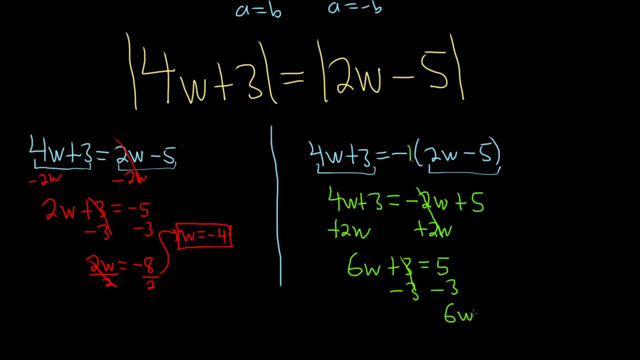 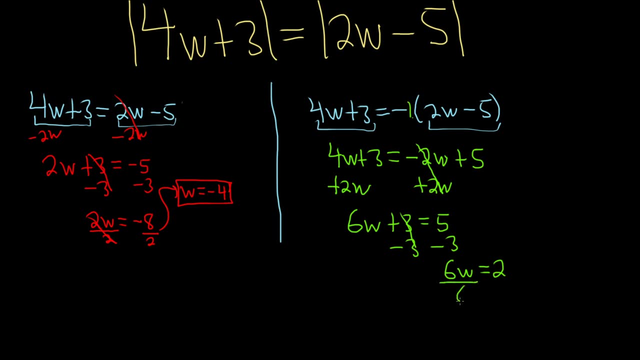 minus 3.. So 6w is equal to 2.. And, as before, it's being multiplied by a number. So to get rid of it we'll just divide. So dividing by 6.. We end up with: w equals 2 over 6,. 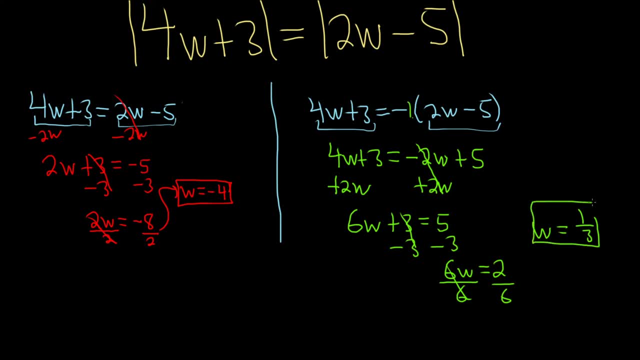 which is the same thing as 1 over 3. So a little bit longer than some of the other absolute value equations. I hope this video has been helpful.